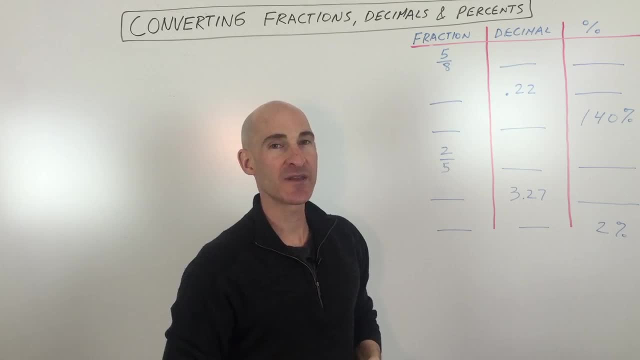 In a fraction, decimal or percentage. how to convert into the other formats? So let's start up here with 5 eighths. We're going to convert from 5 eighths as a fraction to a decimal. Now, when you have a fraction, when you see this division bar, this fraction bar, 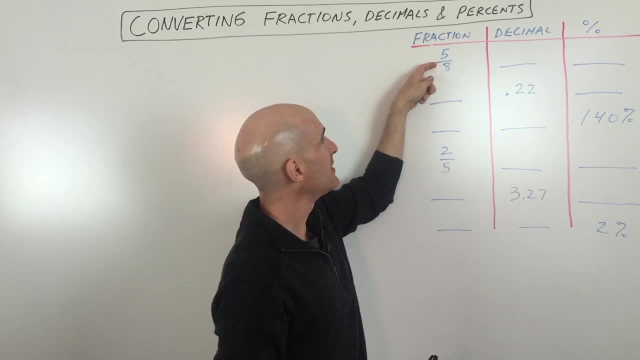 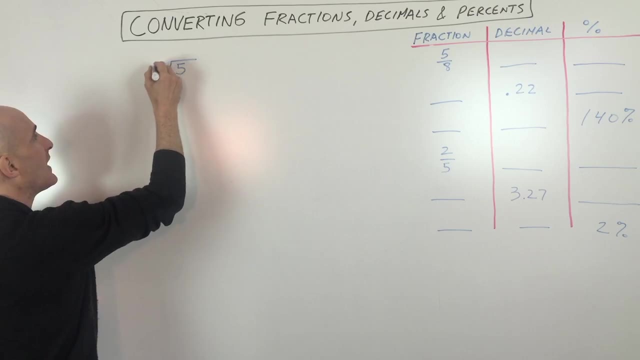 that's really like a division sign. So this is really like 5 is being divided by 8.. So let's go ahead and look at that. So we've got 5 is being divided by 8, or how many times does 8 go into 5?? So if you don't see the decimal point, it's going to be here on the right side. 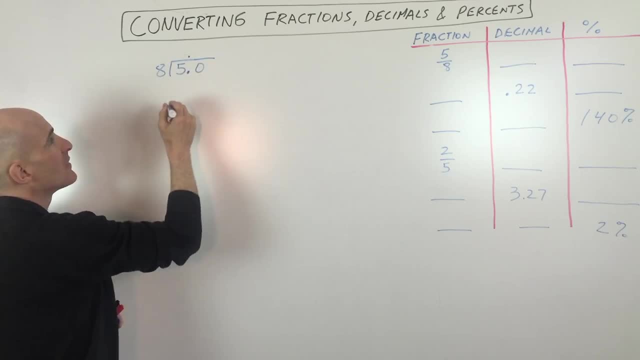 of the number, okay, 5.. And so what we're going to do is we're just going to go ahead and see how many times does 8 go into 5.. Well, it goes in 0 times. Does 8 go into 50?? Yes, it goes into 50. 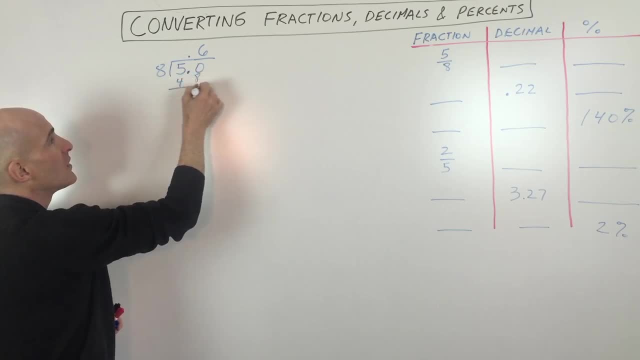 6 times. 6 times 8 is 48.. We're subtracting, we get 20.. Okay, just bring down the 0.. 8 goes into 20 2 times. Okay, we subtract again. bring down another 0.. Okay. 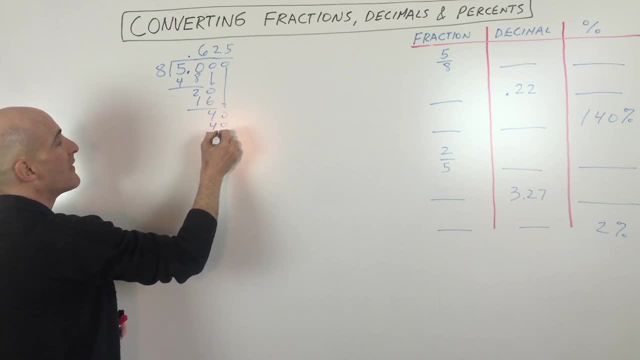 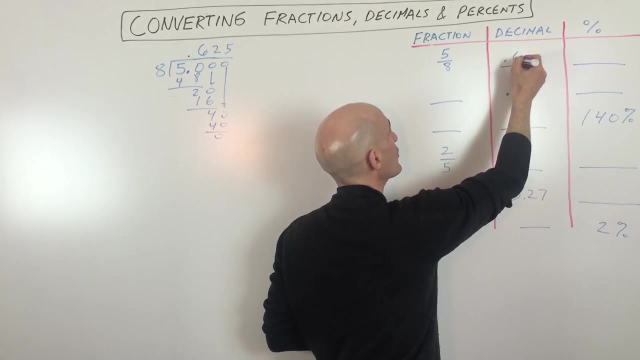 8 goes into 45 times and that goes in evenly. So we have as a decimal 0.625.. So let's go ahead and add that to our chart here: 0.625.. Now to convert from a decimal to a percentage, what we do is we take that decimal point and we move it one, two places. 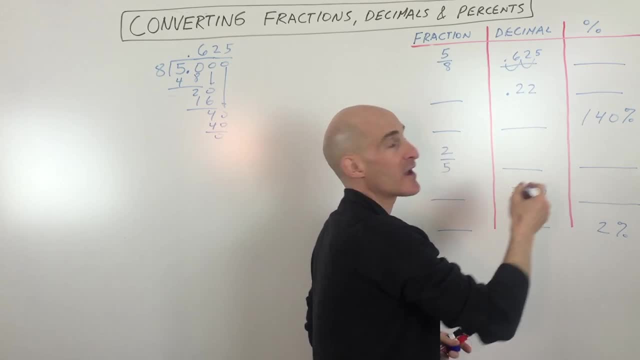 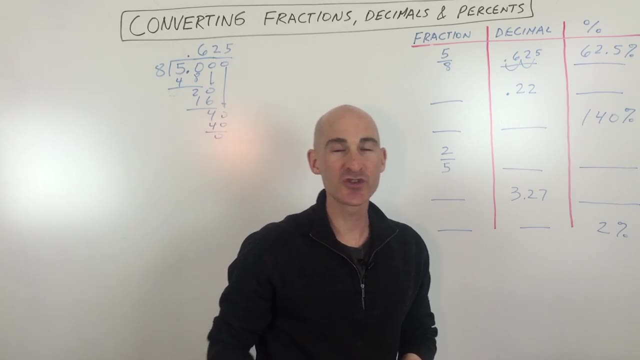 to the right. So it's just like this: one, two places to the right. Now we have 62.5 percent. Okay, so are you with me? so far, We're going to do some more examples Here they're giving us. 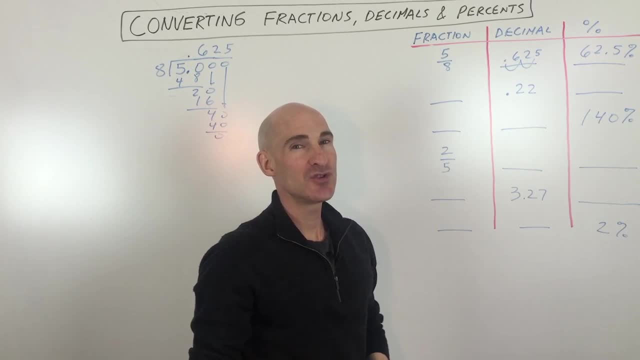 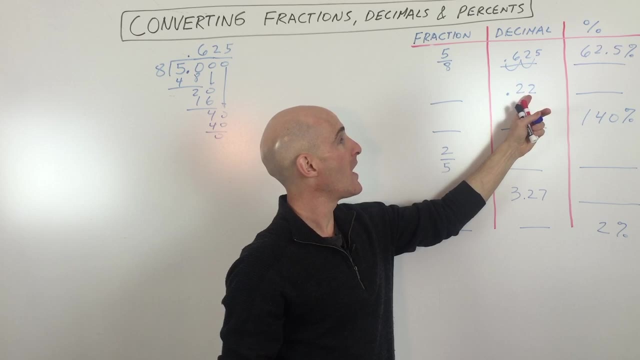 the decimal 0.22.. Now, 0.22 is kind of like a shorthand way, a little bit of a slang way of saying what this decimal is. This is actually 22 hundredths. Now you can see that we want to look at the last place that the number has here, which is the hundredths place, tenths. 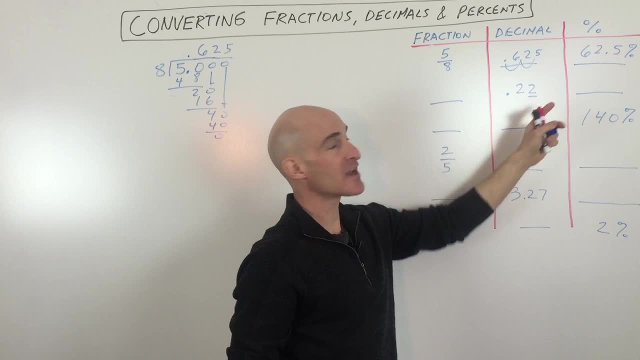 hundredths, thousandths, right? So it's in the hundredths place. So, if you pronounce that correctly, it's 22 hundredths, which means that this fraction is going to be 0.2.. So we're going to say that this fraction is 22 divided by 100.. But you can reduce that further to 11 fiftieths. 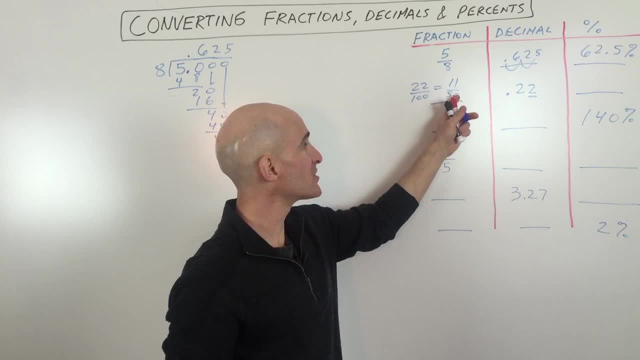 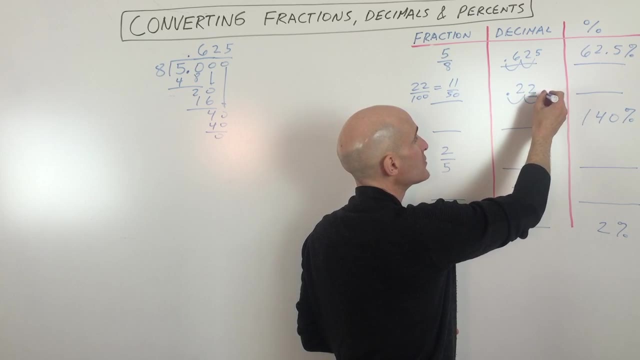 by dividing the numerator and denominator by two. So we're just reducing it to lowest form. Now to go again from the decimal to the percent, that's pretty easy. We just have to move the decimal point one two places to the right, So that's going to be 22 percent. Okay, now in the 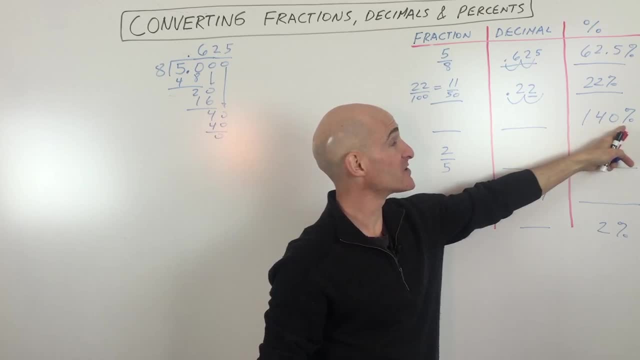 next example: they're giving us a percentage: 140 percent. How do we go from 140 percent back to a hundred and forty percent? Well, we're going to do a little bit of a math test here. We're going to do a decimal. Well, here, what we're doing is we're actually going to be moving. 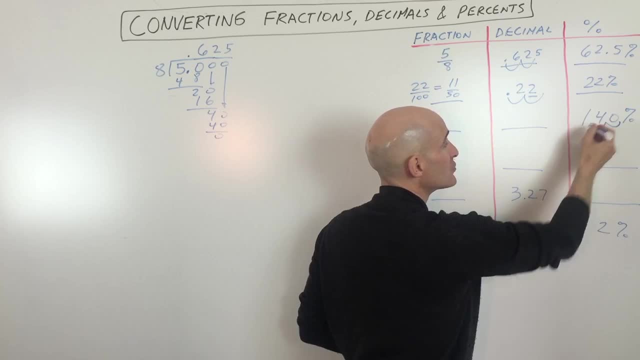 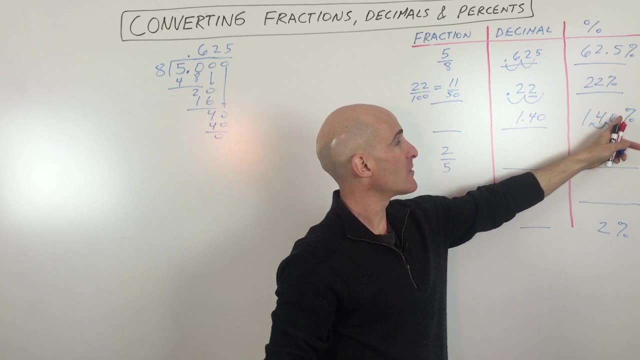 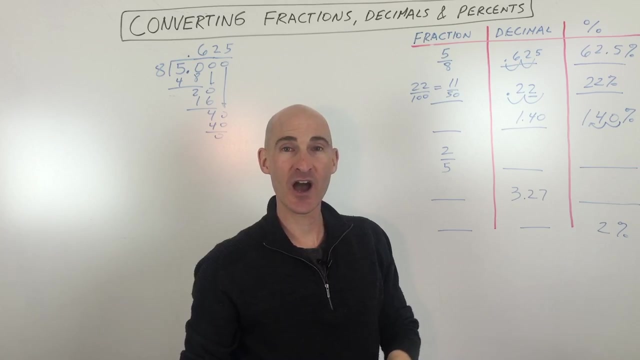 the decimal point to the left two places. So this is actually 1.40, or you could just say 1.4.. Another way to look at it is percent Per means. divided by cent means hundred, like a hundred cents in a dollar, a hundred years in a century, a hundred feet on a centipede, and so on. So per. 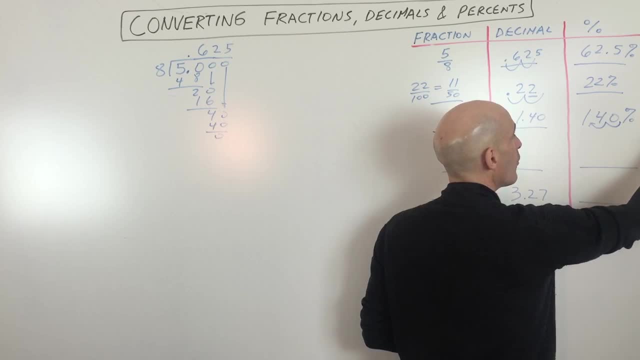 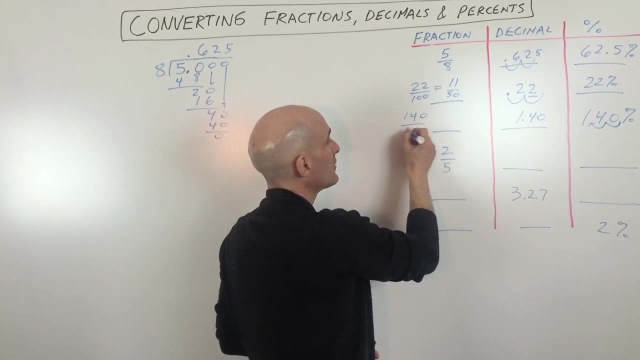 cent. you can think of this as 140 per 100.. And that'll also help us to convert this into a fraction, okay, which is 140 over 100, and we can reduce that to 14 over 10,, which is 7 over 5, or, if you want to write it, as a mixed number. 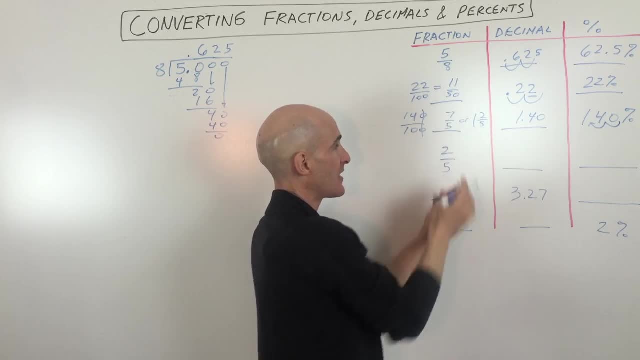 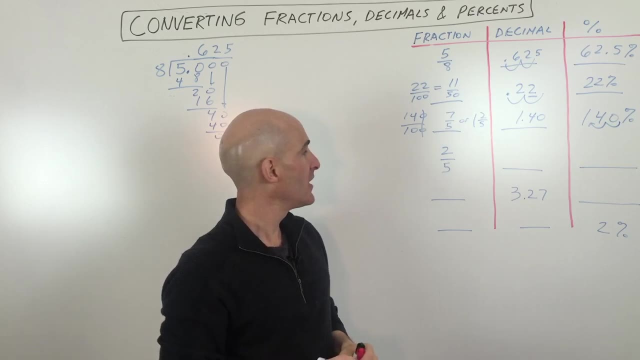 one and two-fifths. Five goes into seven one whole time, with two left over. so one and two-fifths. Okay, let's just do a few more examples. I hope you're enjoying these videos. Let's take a look at this example here: two-fifths- We want to convert that to a decimal. 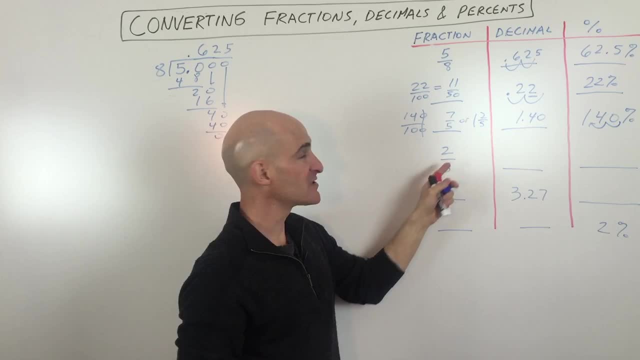 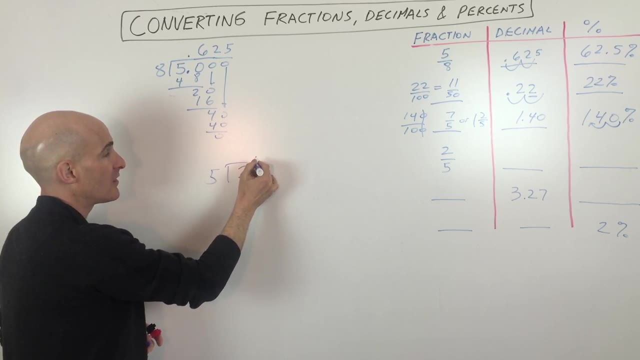 right. So two divided by five. So the fraction bar means divided by. so let's go over to here. Two is being divided by five. Five goes into two, zero whole times. Okay, five goes into 20,. four times Four times five is 20, with zero left over. so we can see our decimal is going to be. 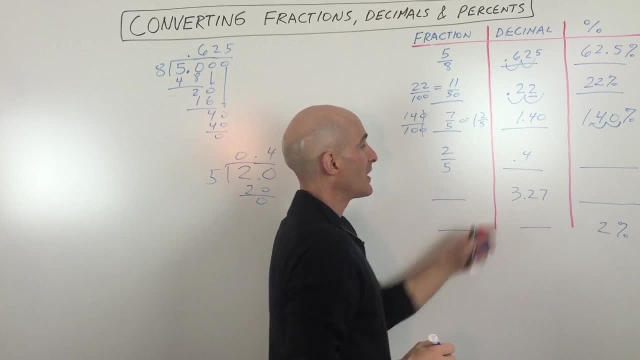 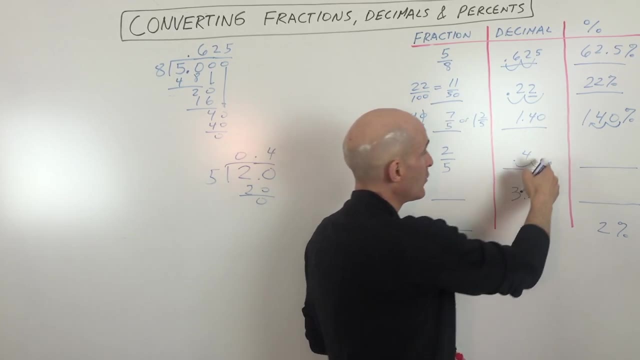 0.4.. So this is 0.4.. Okay, now to convert from the decimal to the percent. we're going to move that decimal point one, two places to the right. We're going to have to put a placeholder here, since there's not a number there. so that's going. 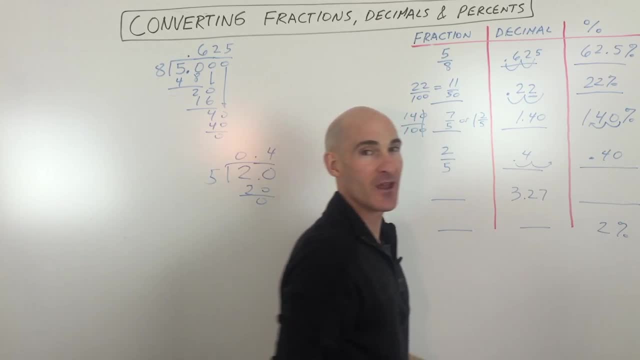 to be a zero, so it's going to be 0.40.. Okay, two more to go: 3.27.. Should we convert it to a percent or to a fraction? Let's do the percent first. So we're going to move the decimal two places to the.